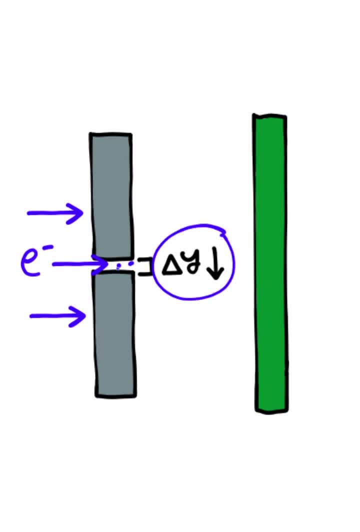 By narrowing this slit you decrease the uncertainty for the position of the electron, but you'll increase the uncertainty in the momentum. so you'll actually see a wider spread, because the electrons will have more uncertainty in their movement. So it's a bit counterintuitive, but that's the basic idea of the.